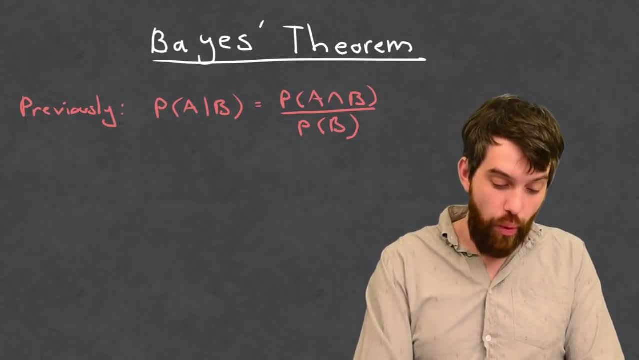 of B. Now I'm going to rearrange this, I'm going to go the other way around. So if I have this, I can also, therefore look at what the So, if I have this, I can also, therefore look at what the 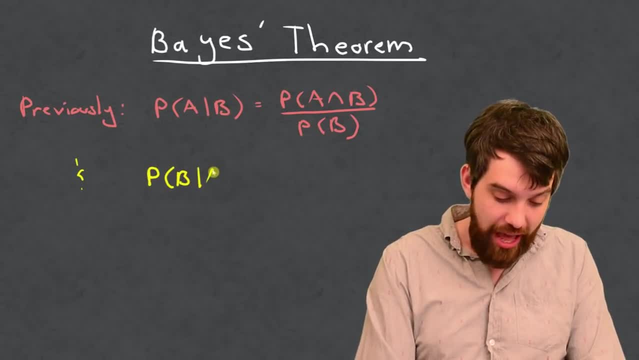 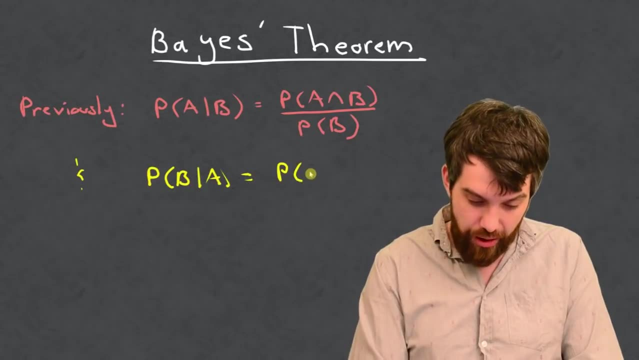 happens if I take the probability of B given A. So the same thing. but just flip the other way around and by comparing these two, it just has to be the probability. now it's B intersect A. Note that that doesn't matter: A intersect B and B intersect A. I can flip. 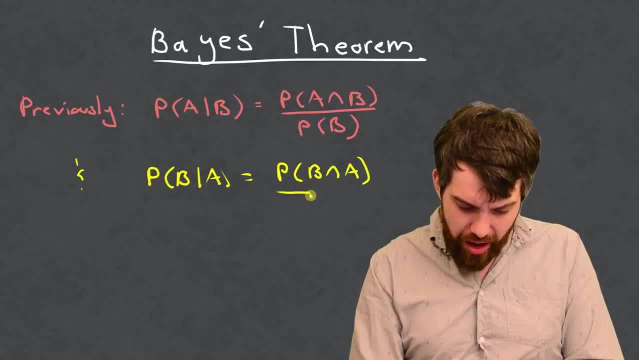 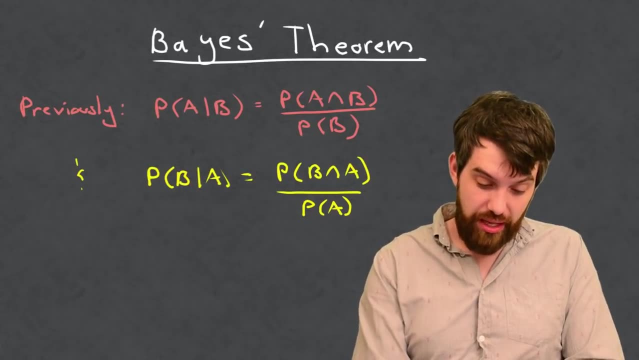 those around it doesn't make any difference. And then now it's all divided out by the probability of A. So we have these two different components, and you'll notice that there's this portion, the numerator, that these two things are indeed going to be equal, So I can take the one. 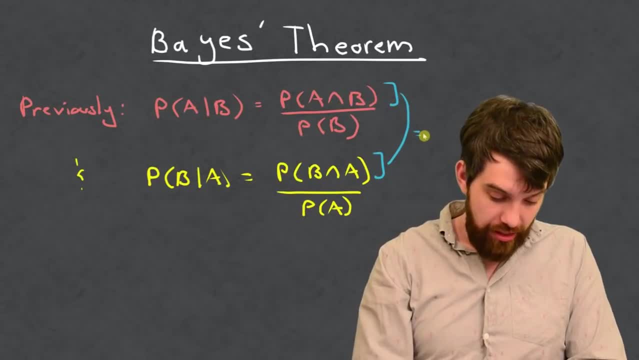 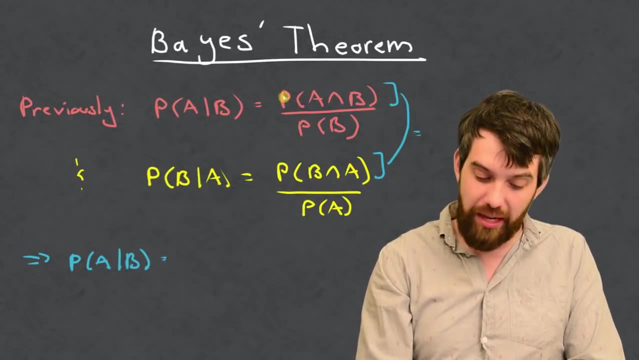 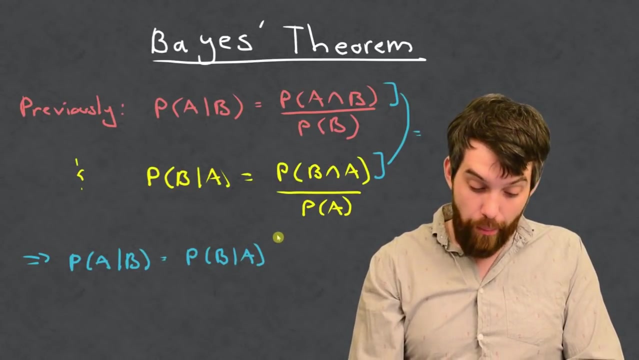 the bottom one and I can substitute it into the top one. So what that's going to give me is that the probability of A given B is equal to- well, the probability of the intersection. but I'm going to rewrite that as the probability of B given A multiplied by the probability. 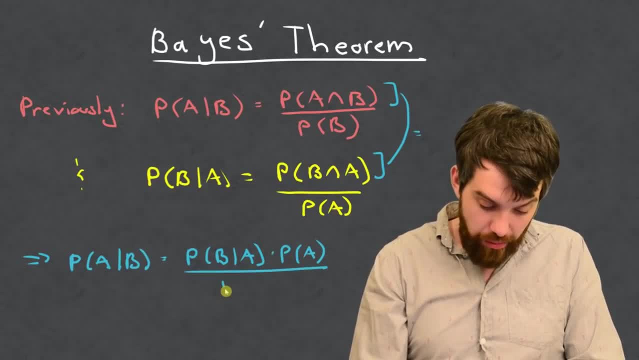 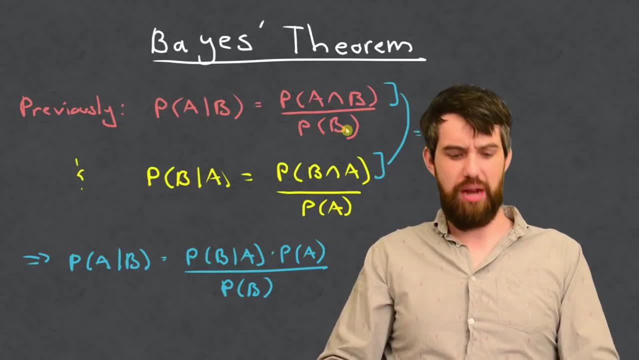 of A and then all divided out by the probability of B, as I have down below, On the bottom right here. So what I want you to note about this formula, this is going to be Bayes' theorem right here. this is what it is, at least in the single case where we've 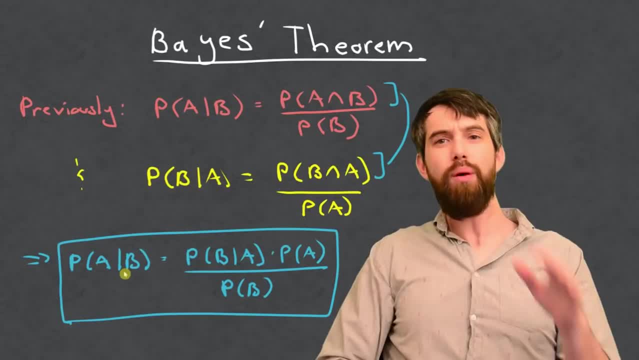 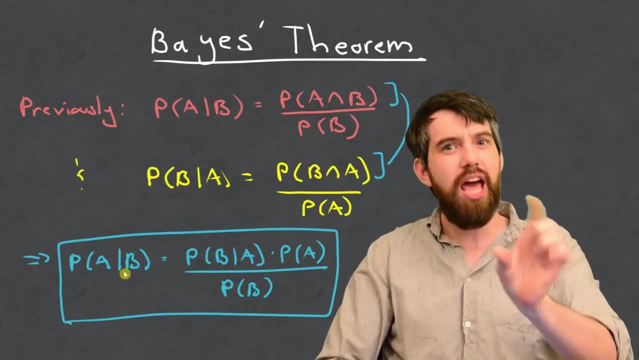 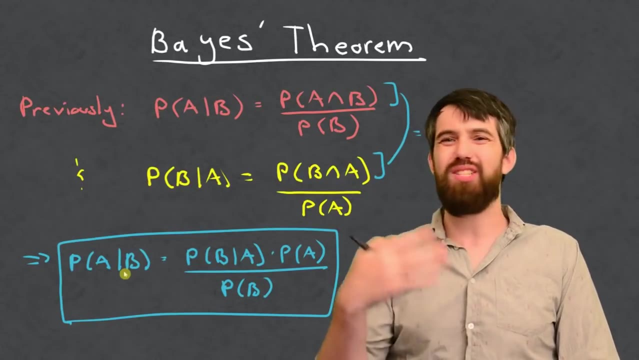 only got one B that we're interested in, and what we have here is that we can sort of alternate the A given B or B given A. We can change that rule around by multiplying by this particular ratio the probability of A divided by the probability of B. Now, the reason why this: 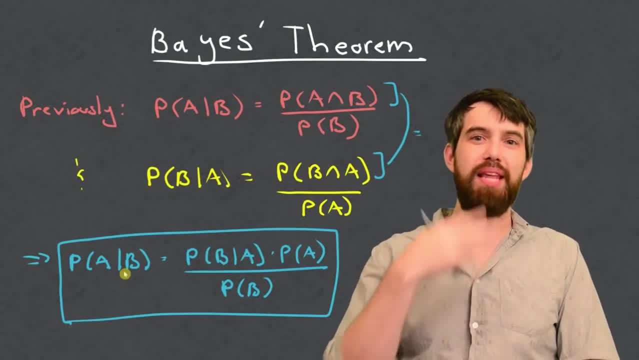 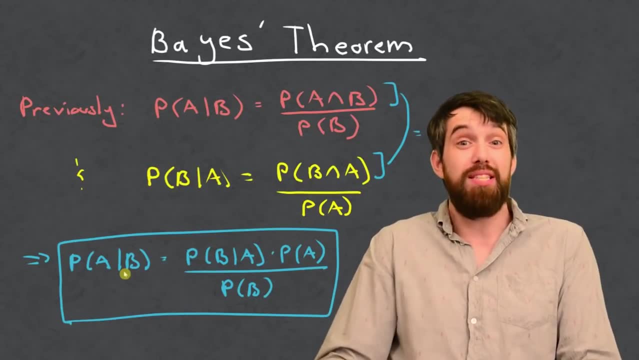 is so helpful is that sometimes computing the probability of A given B is easy, and sometimes the probability of B given A is easy. Sometimes they're both easy, but in any scenario where one of those two is easy to compute, maybe you can go out in the real world and collect some data and 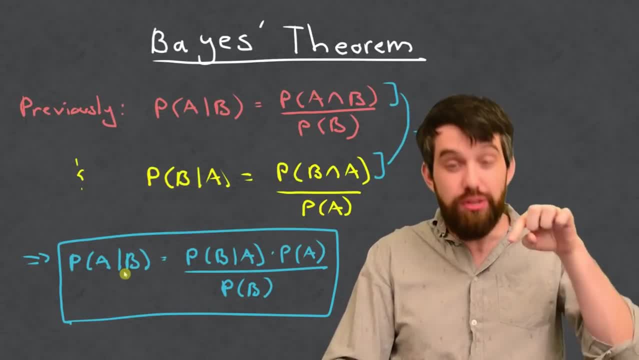 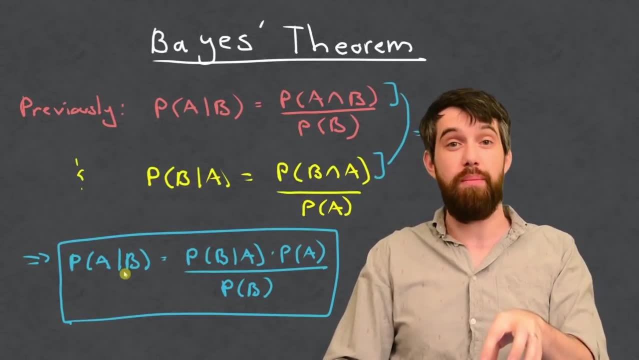 figure it out, but that the other of the two is a little bit more challenging. you can use this formula to convert them. You can get from the one conditional probability to the other conditional probability that are related by Bayes' theorem. So let's look at an example we've seen before in the previous video. 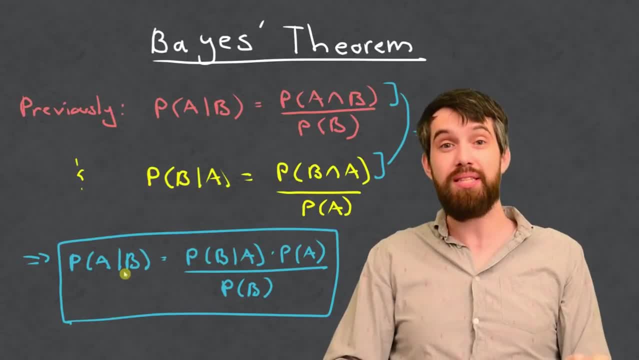 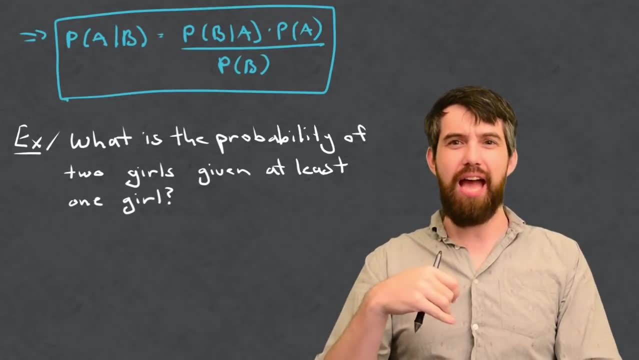 but we're going to investigate it in the context of this Bayes' theorem. So the example was: if you have a couple and they got two different children and you're asserted that at least one of those children is going to be a girl, then what's the probability? 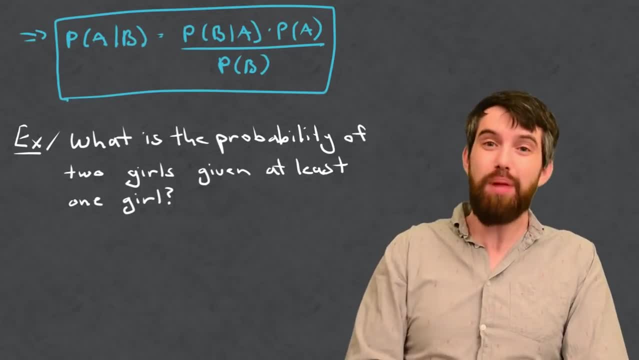 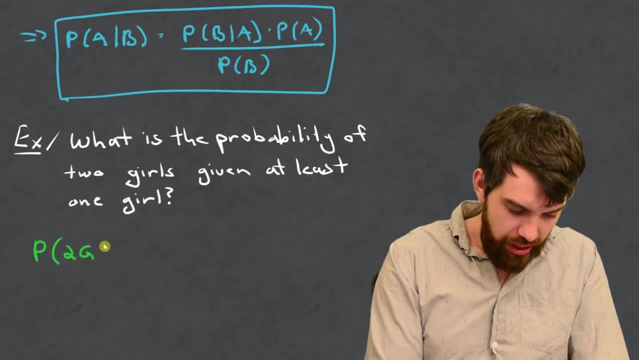 that both of the children are going to be a girl, So let's put this into the formula. So I'm asking, in effect, I want to know what is the probability of the two girls, given that we're going to have at least non. 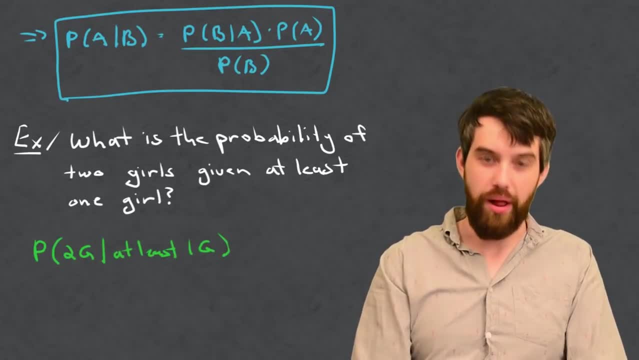 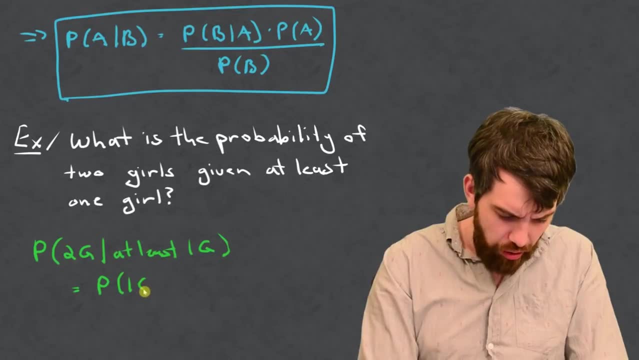 Haloẩ in Video. in Video: least one girl. Well then, this by the theorem tells me that this is the probability, and I'm going to abbreviate even more and just go all the way down to one girl. I mean at least one girl, but I'll just write 1g, given that I have two. 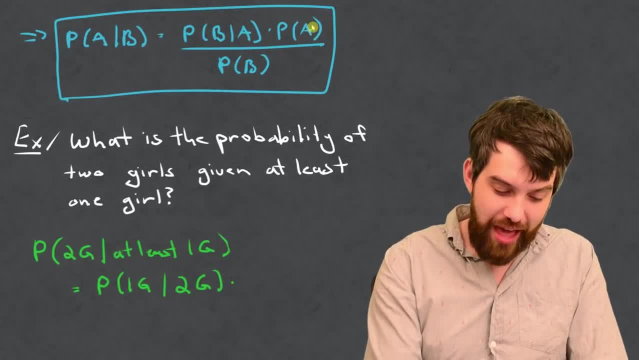 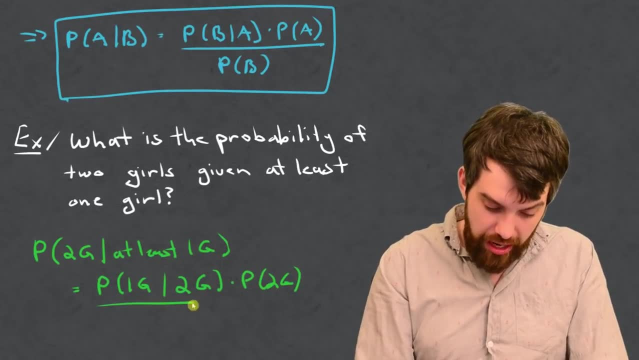 girls multiplied by P of A- here P of A is the first thing- so multiplied by the probability of two girls, and then finally divided out by the probability of B. so this is the probability of at least one girl, which I've abbreviated to. 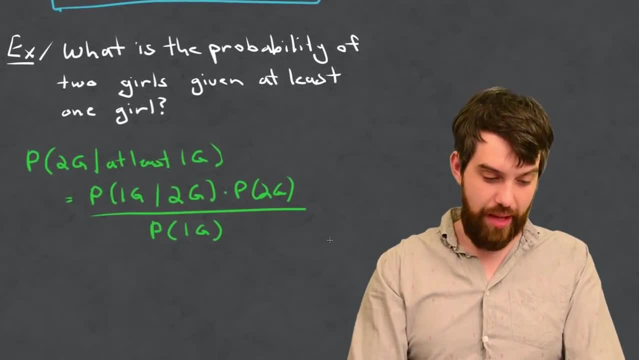 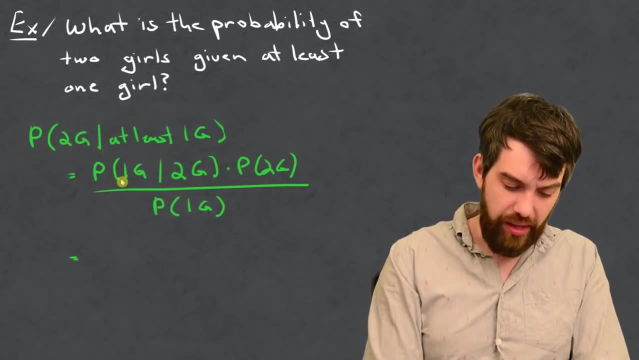 be the probability of 1g. Alright, so we have this computation, so how can we actually go and evaluate it now? Well, let's look at this conditional probability, the probability of having one girl, at least one girl, given that. 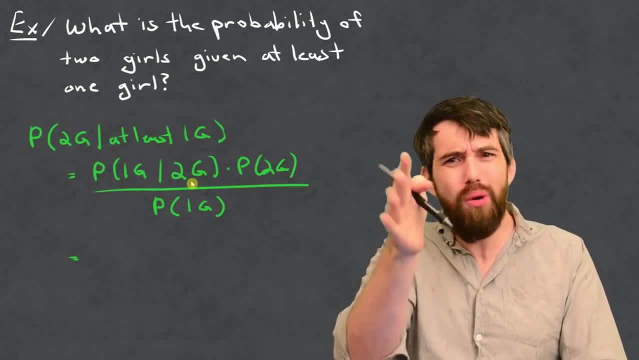 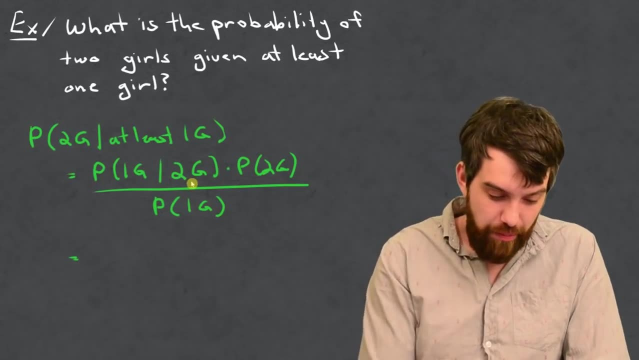 you know that there's two girls, But if you're being told that there's two girls, then the probability of having at least one girl is 100%. If you have two girls, you have at least one of them. So the P of 1g, given the 2g, is really really easy to compute. It's 100% or it's just? 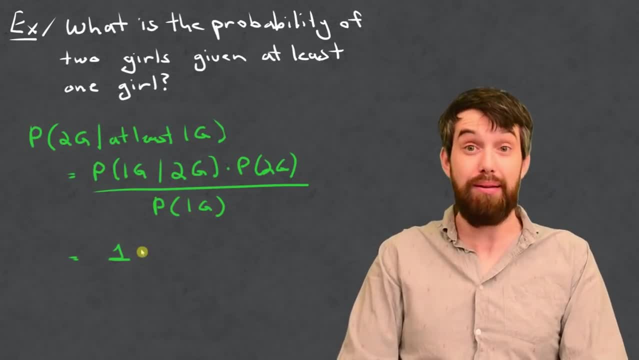 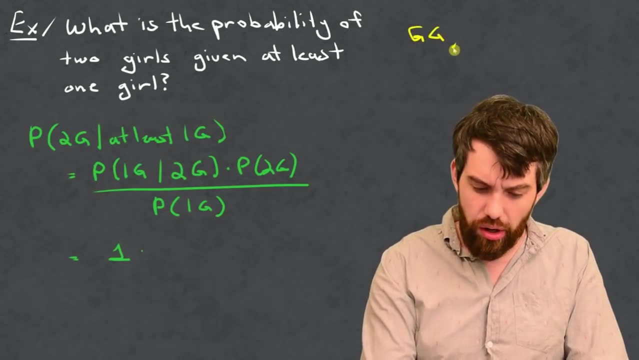 the value of 1.. I don't have to do anything. Okay, well, that was nice. What about the probability of there being two girls? Well, you might remember that the four cases are: you could have a girl-girl, you could have a girl-boy, you could have a boy-girl and you could have. 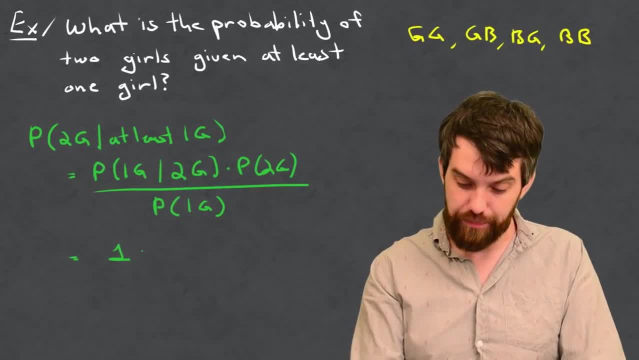 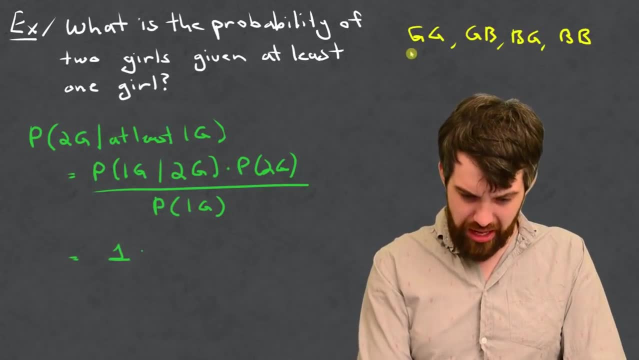 a boy-boy. There were sort of four different sort of possibilities, But then if we're going to investigate this, we want to investigate what's the probability of having two girls. well, there's only one of those four possibilities, So this is just going to be the value of a quarter. 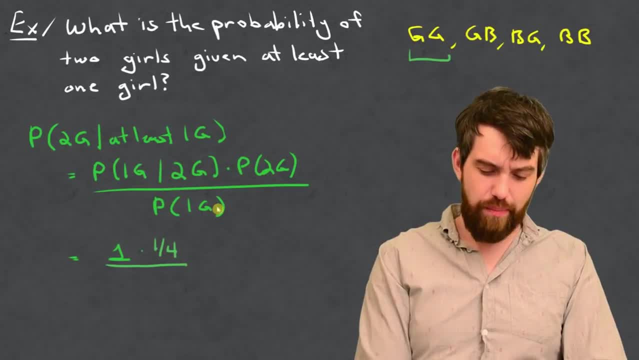 And then I divide out by the probability of at least one girl. Well, this one has a girl in it, that one has a girl in it, that one has a girl in it. there's three of them that have a girl. 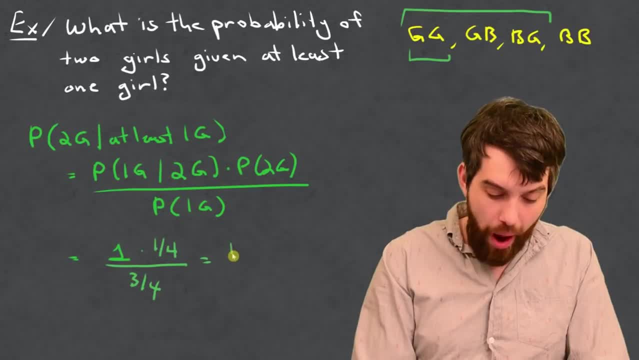 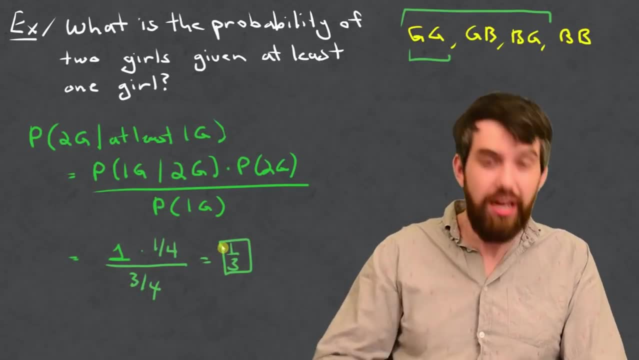 so three-quarters. In other words we get one-third, Which is the same value that we computed just by pure conditional probability. but we verified that it works using Bayes' theorem. That illustrates at least some motivation at Bayes' theorem. 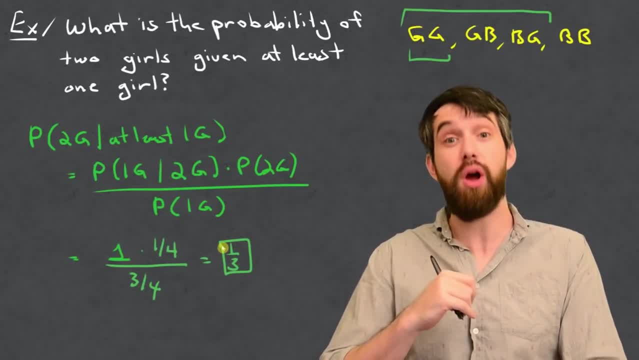 This is likely going to be true and useful, presumably in other contexts beyond this. 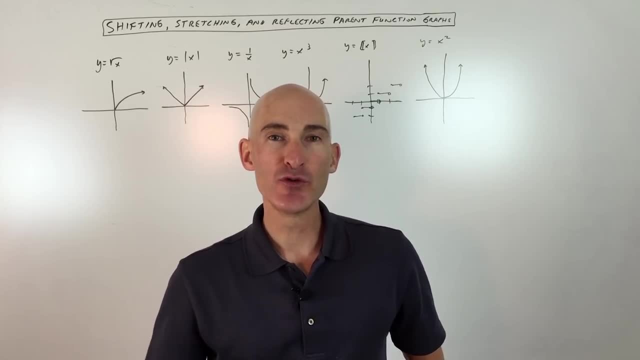 Hi, this is Mario, with Mario's Math Tutoring, coming to you with another math video to help you boost your score in your math class, improve your understanding and, hopefully, make learning math a lot less stressful. So what we're going to talk about in this video is how to stretch, shift, translate, reflect all the different types of transformations that you can do with parent functions. 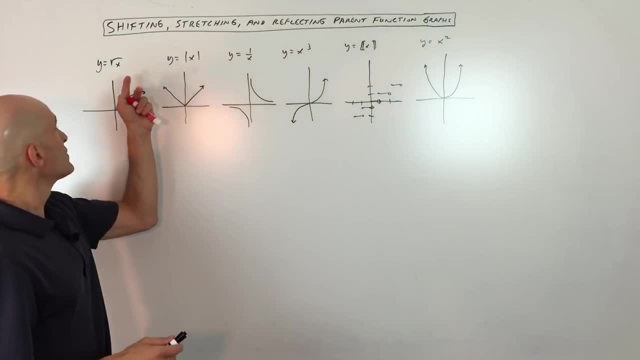 So let's get right into this video and look at some examples. So first of all, you want to familiarize yourself with a lot of these basic graphs If you recognize the basic shape of the graph and the basic equation. that's the starting point. 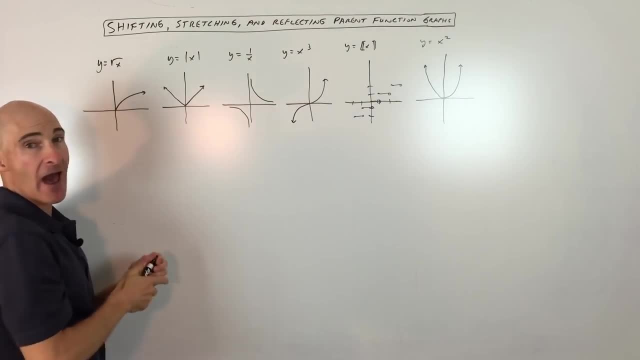 So let's just go through them real quick. This is the square root function and it looks like half a parabola on its side. This is the absolute value function and it looks like a real sharp V with the vertex at the origin.